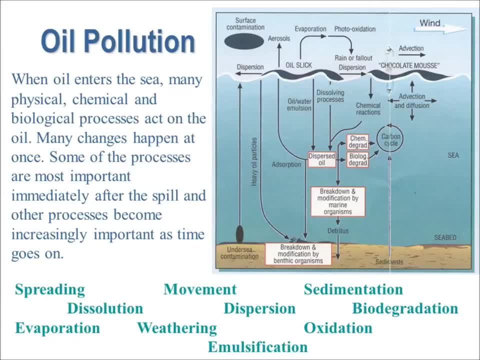 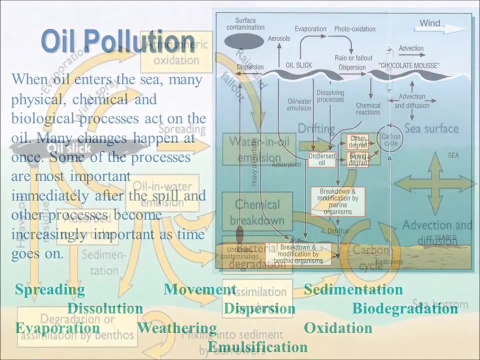 The slick or spill spreads over the surface of the water due to the force of gravity, Spreading decreases steadily as time passes. Dissolution Occurs when the water-soluble components of oil break down into the large volume of water surrounding the spill. 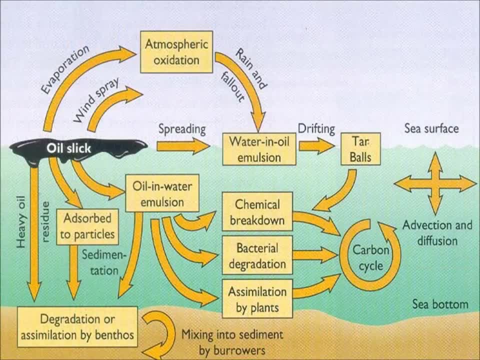 Only a very small percentage of oil dissolves Sedimentation. The force of gravity will cause some of the oil to travel through the water and settle on the bottom Movement. An oil spill will move in the same direction and at a similar speed as the water. 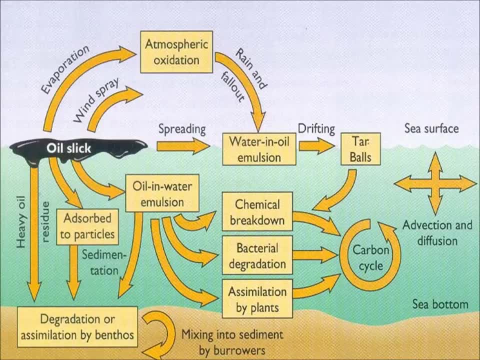 It is moved by currents, tide and wind. Biodegradation: Many species of marine microorganisms or bacteria, fungi and yeasts feed on the compounds that make up oil. Hydrocarbons consumed by these microorganisms can be partially metabolized or completely metabolized to carbon dioxide and water. 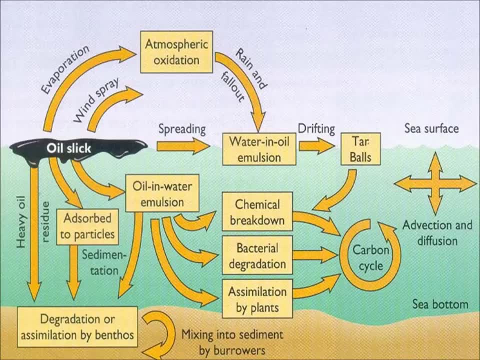 Oil can be metabolized to carbon dioxide and water. The rate of biodegradation depends on the temperature of the oil in water mixture. Evaporation Causes some of the oil to transfer to the atmosphere. Lighter hydrocarbons evaporate more rapidly than heavy component. 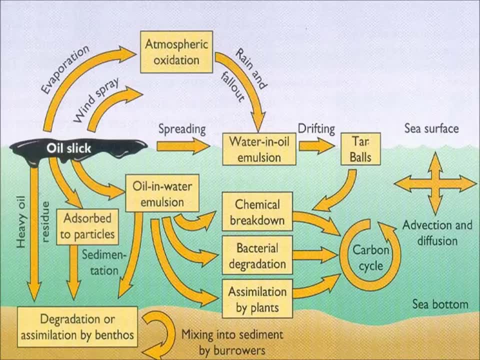 Weathering Is a progressive series of changes in oil characteristics caused by physical, chemical and biological processes. The rate of weathering is highly dependent on the type of oil spilled. The lighter it is, the faster it is likely to weather. Temperature changes in water and water mixture cause some of the oil to transfer to the atmosphere. 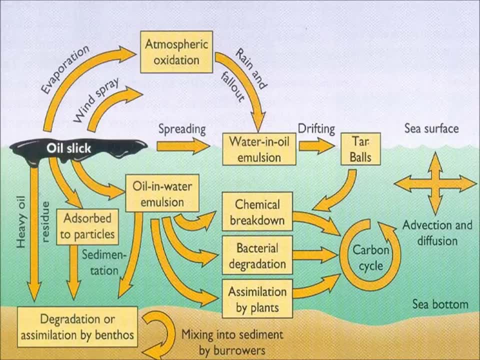 is likely to weather dispersion. the spilled oil is spread into the upper layers of the water column by natural wave action. oxidation: the chemical combination of hydrocarbons with oxygen, is known as oxidation. oxidation is slow compared with other weathering processes. emulsification is the combination of two. 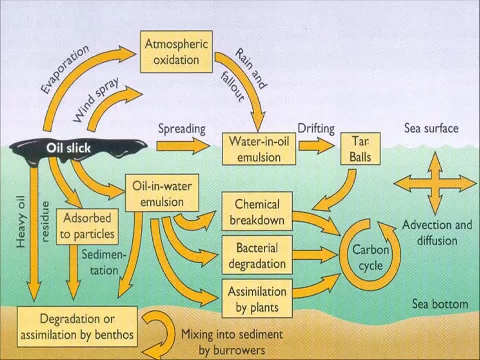 liquids once suspended in the other. in the case of oil, the emulsion can be either oil in water or water in oil. milk is an oil in water emulsion. butter is a water in oil emulsion. both types of emulsification require wave action and occur only for specific oil compositions. water in oil emulsions are extremely 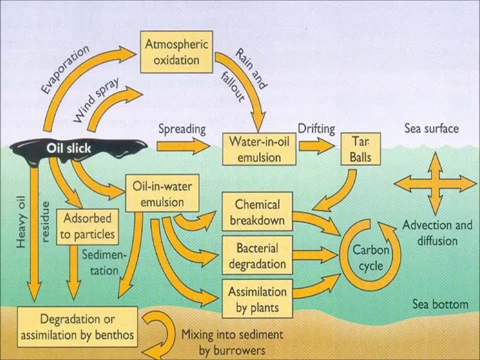 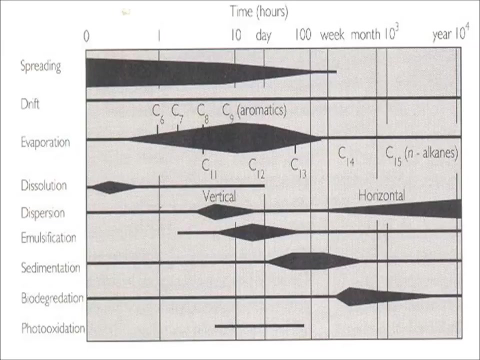 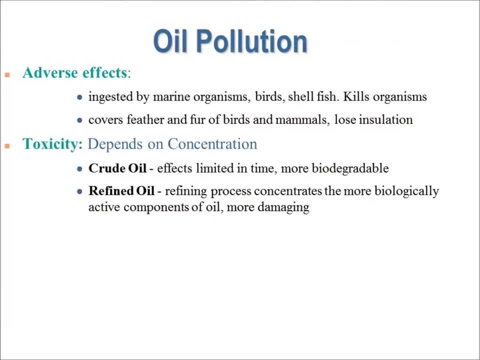 stable and may persist for months or years after a spell. water in oil emulsions containing fifty to eighty percent water are most common and have a reddish brown color and grease like consistency. they are sometimes called chocolate mousse because of their pudding like appearance. they are mostly made of chocolate and then separated into two or three. 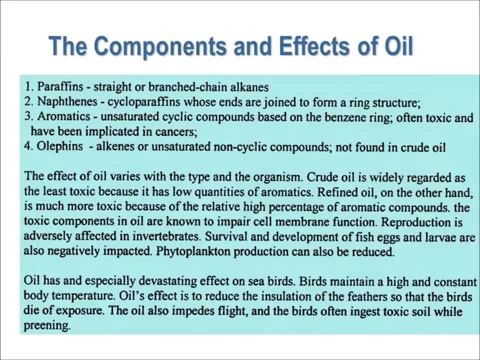 layers and then spread to make water in the water column. this is very common and it also helps in the development of the water column into a water column because it gives a much larger amount of water into the water column so water is able to absorb water in a more 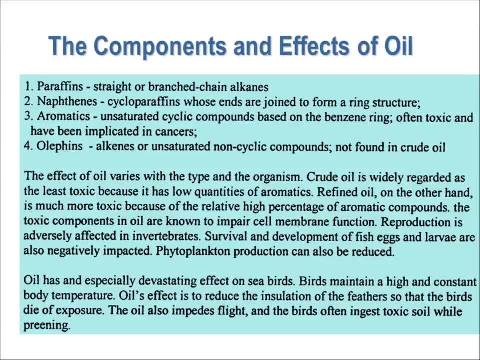 fluid way, and this is very hot in hot weather or any time period. so that's how it works. it's also known as the same as the water column. chose both methods, one already have the same reaction and this is the same as the water column, and it's now is combined with the water column in one. 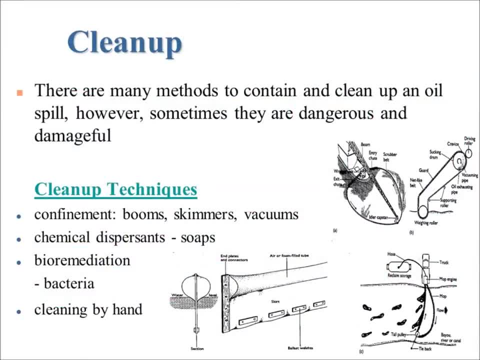 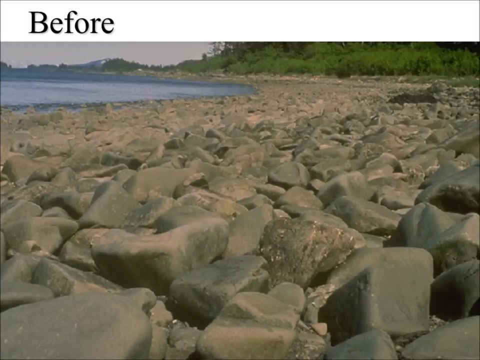 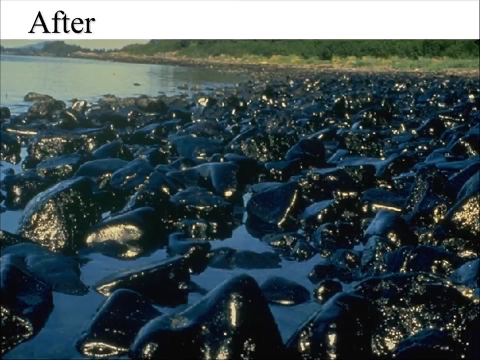 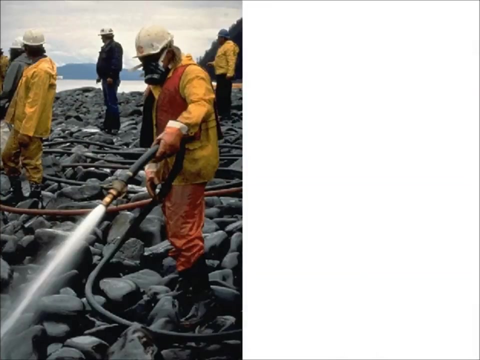 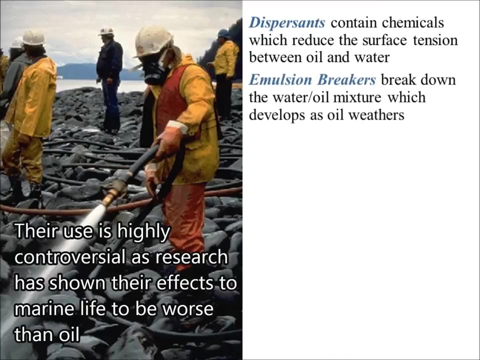 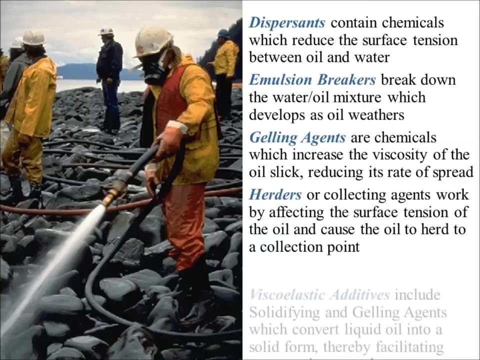 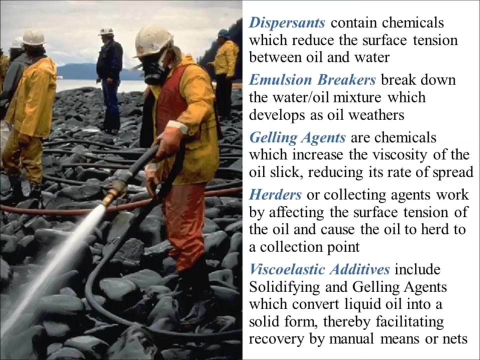 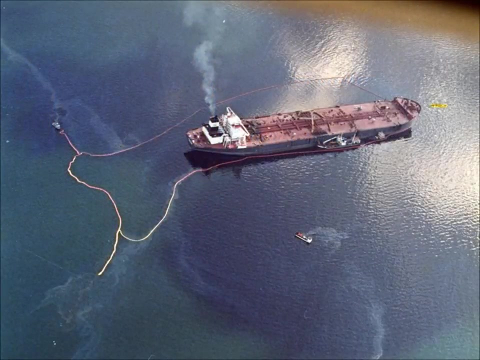 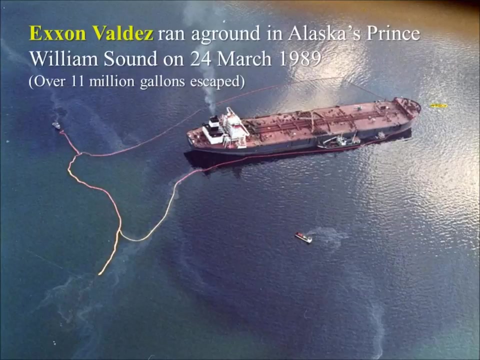 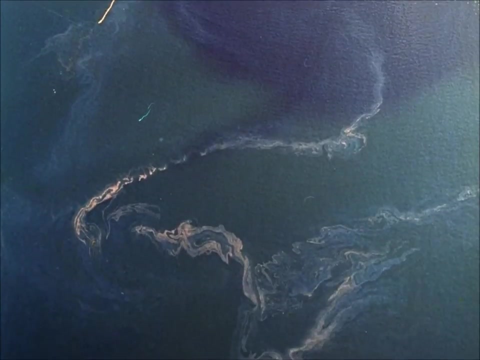 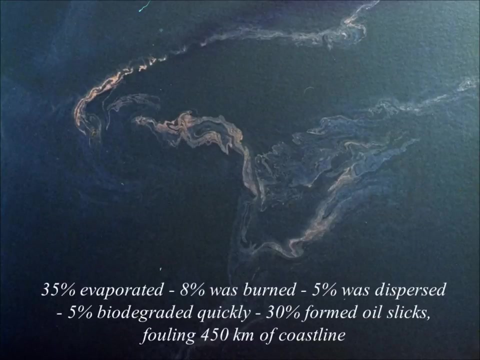 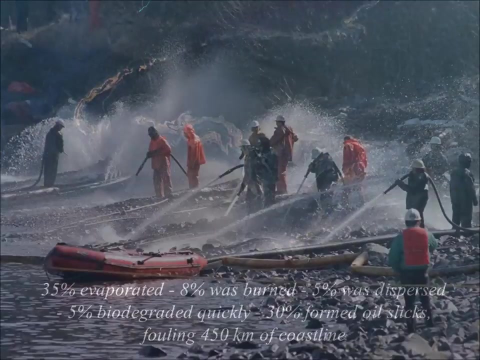 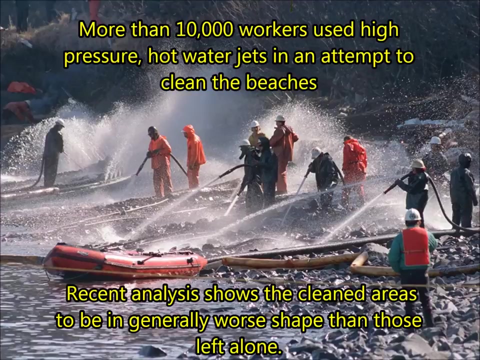 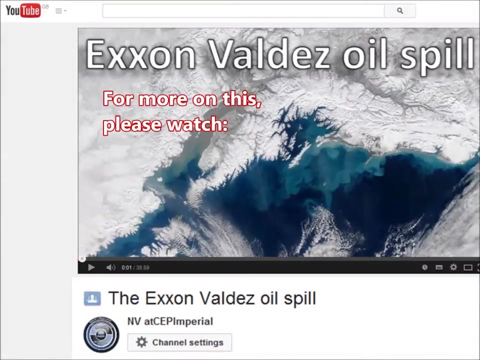 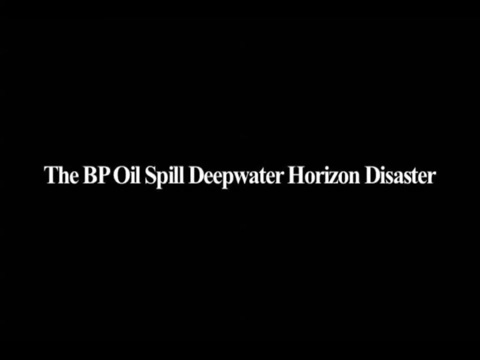 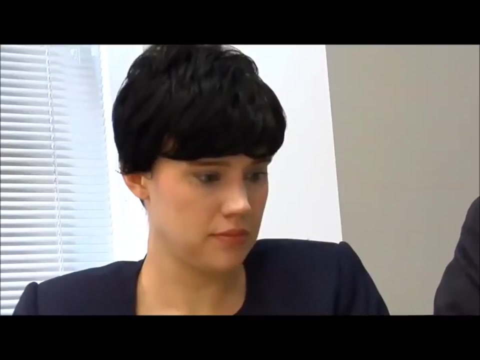 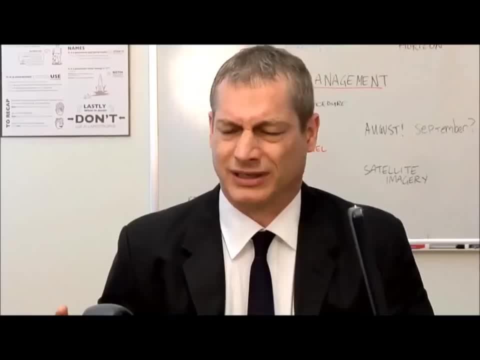 It's a small spill on a very large table, Sir. I think we're underestimating just how much coffee was spilled. Yeah, that's a lot of coffee. Well, we'd better hurry up, because it's almost reached my laptop. 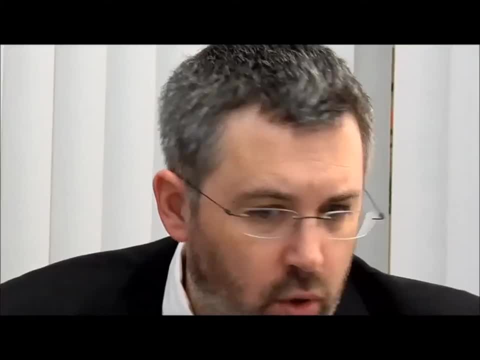 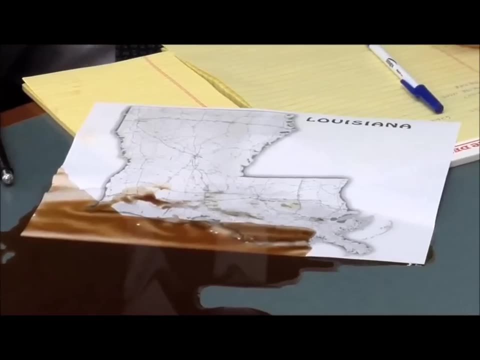 Calm down, Calm down. It's also going to destroy all the fish. Oh boy, Okay, Boom, Look at that, My God, it's encroaching on my map of Louisiana. Okay, Okay, Look, Oh no. 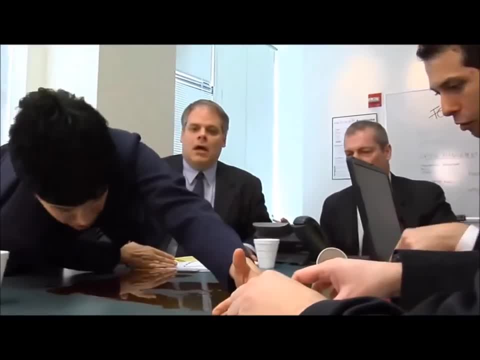 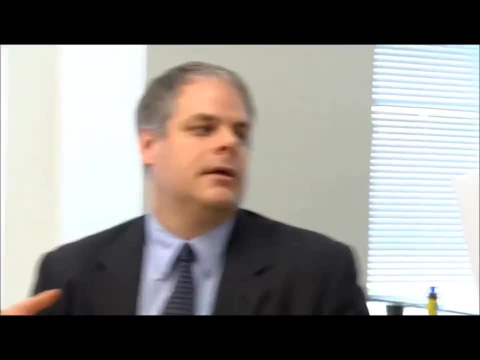 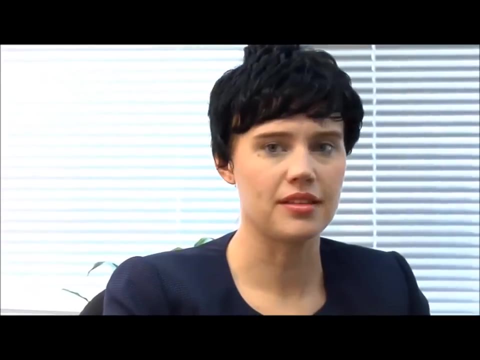 It's the laptop. Okay, I'm sorry. Oh, no, It's the laptop. Wait, Wait, Wait, Wait, I've got a brilliant idea. Oh, Okay, Jones, you've got to hurry up. I think the public is getting suspicious.